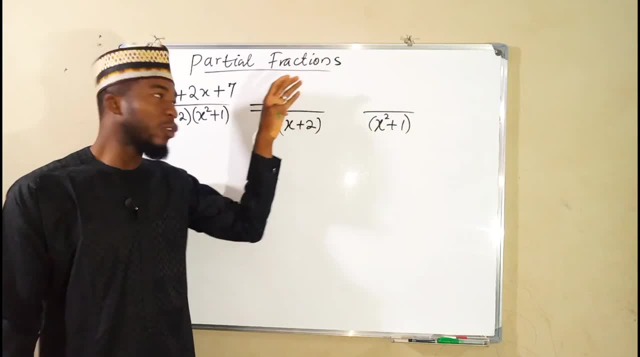 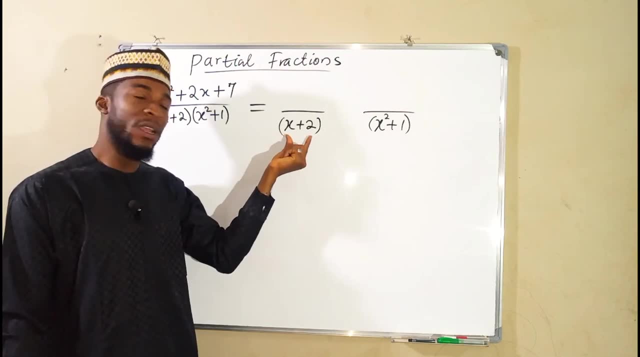 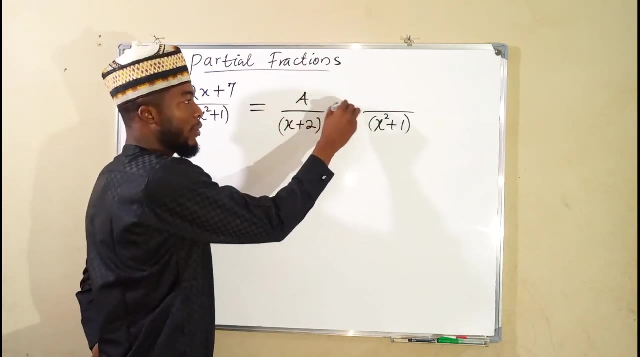 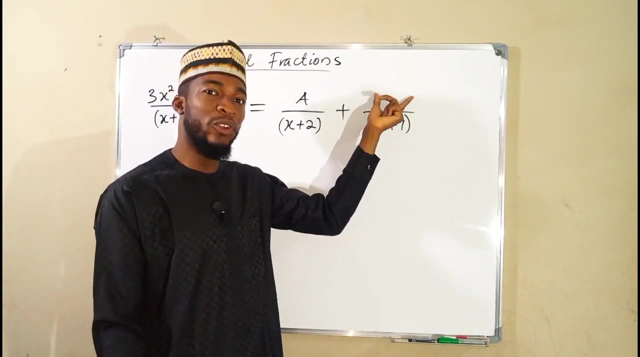 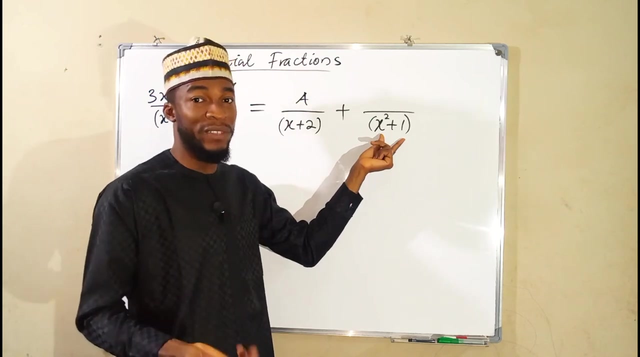 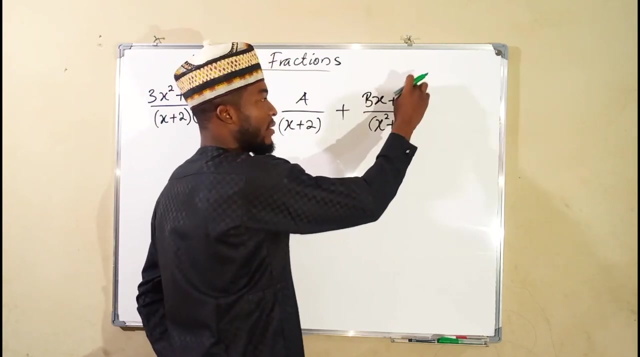 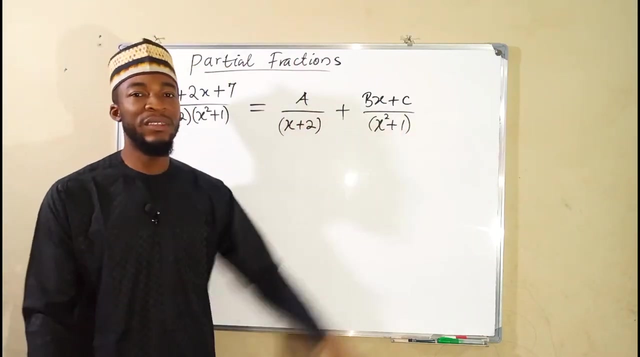 I told you the corresponding numerators are going to be a polynomial of one degree less than the denominator. This is a linear factor. Therefore, the numerator is going to be constant. So we can name that constant as e. Then plus the other fraction. This is a quadratic factor. Therefore, its numerator is going to be a polynomial of one degree less than this. And one degree less than this is going to be a polynomial of degree 1. So we have something like this, bx plus c, where b and c are constants. So now having obtained this, we are going to find the values of a, b, and c. To do that, let us multiply each of these fractions by these two factors. 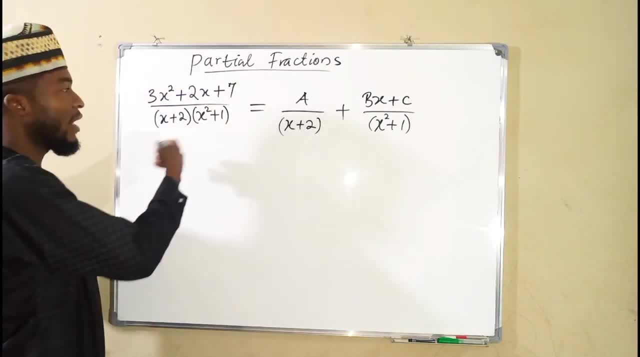 If you multiply the left-hand side by these two factors, they are going to be eliminated, leaving only the numerator. We have 3x squared plus 2x, then plus 7. 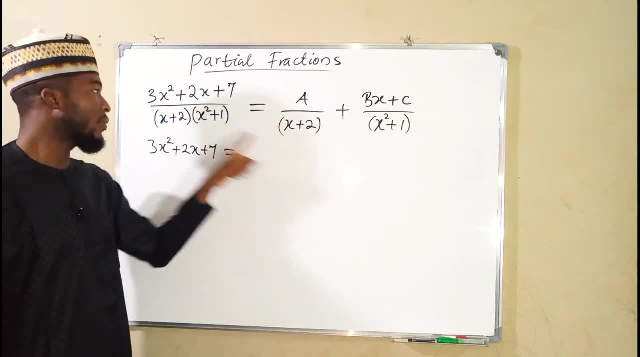 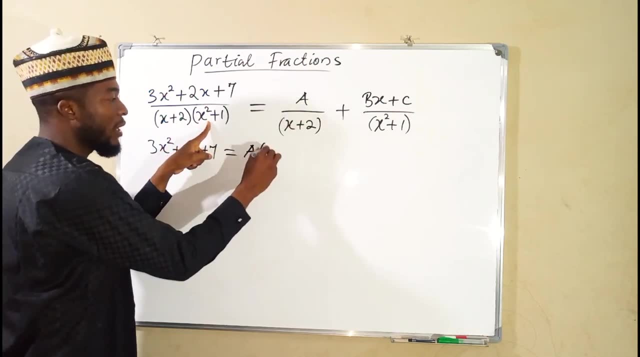 To the other side, if you multiply this with these two factors, this and this will cancel out, leaving only this time this. So we have a multiplied by x squared plus 1. Plus. 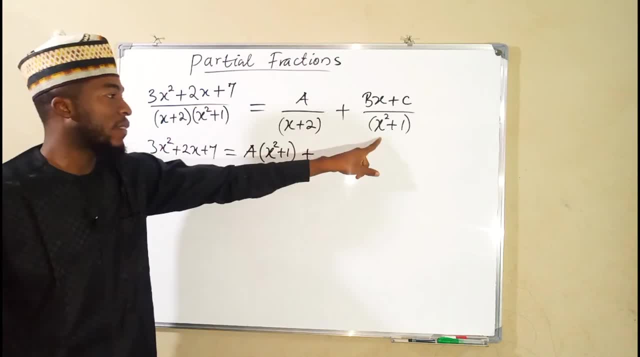 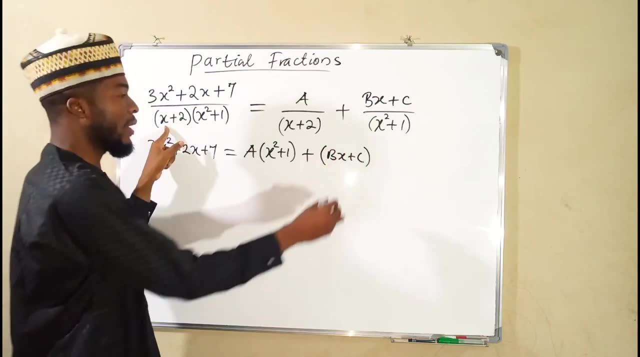 If you multiply this, by these two factors, this will eliminate this, leaving only this. So we have bx plus c multiplied by x plus 2. 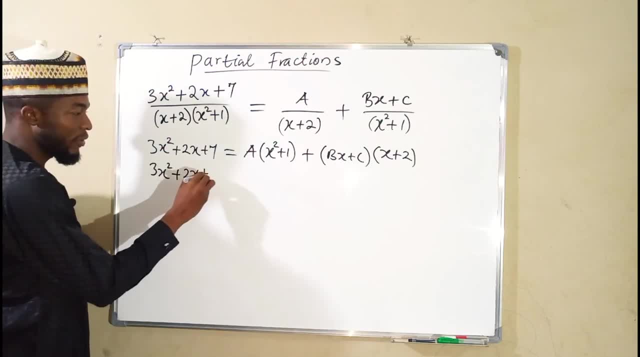 3x squared plus 2x plus 7 from the left-hand side is equal to, we are going to expand all this. 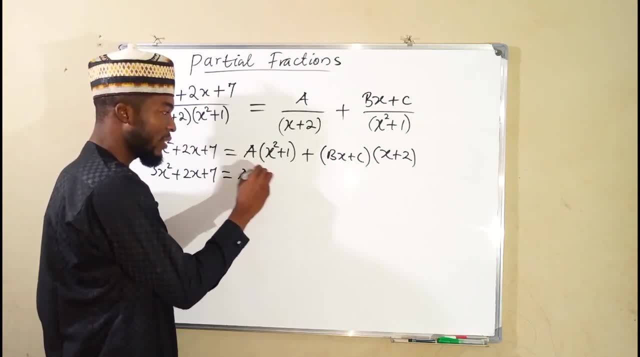 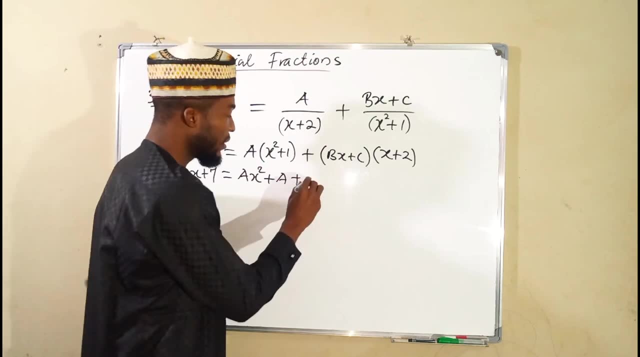 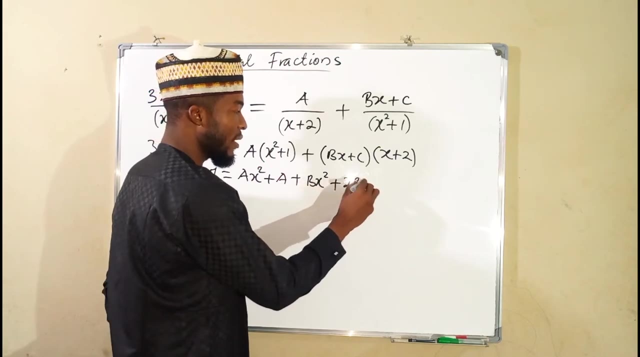 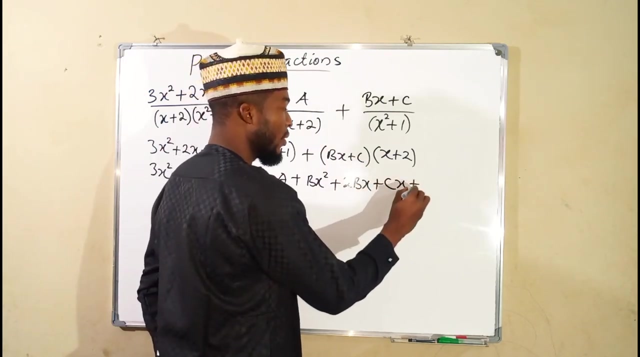 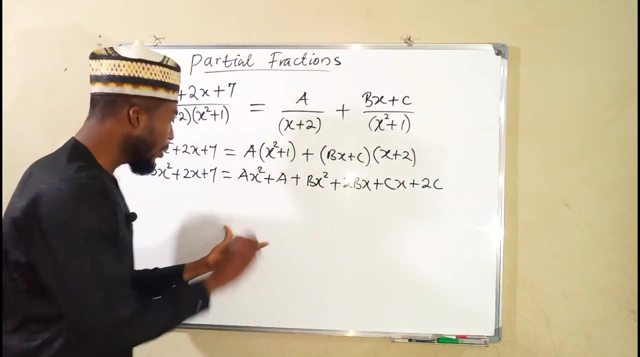 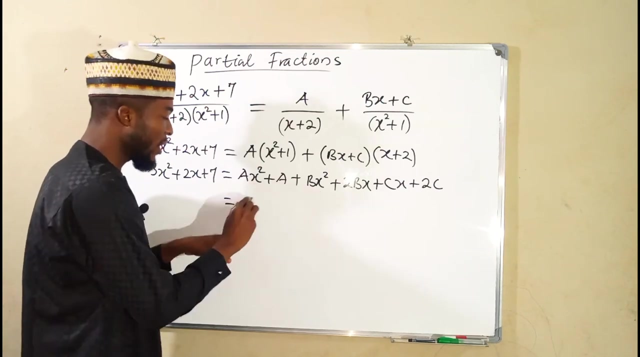 This time this is going to be ax squared. This time this is going to be a. Then plus bx times x is going to be bx squared. bx times 2 is going to be 2bx. Then the other term, we have c times x, cx. We have c times 2, 2c. Now all those with x squared, we are going to connect them together. But we can directly factorize. You can see these are the two terms that contain x squared. a x squared, bx squared, so we can say a plus b. 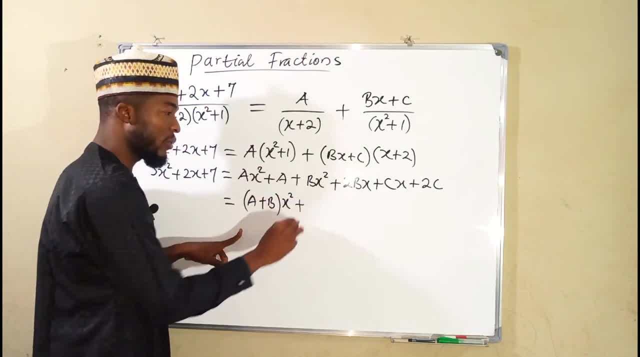 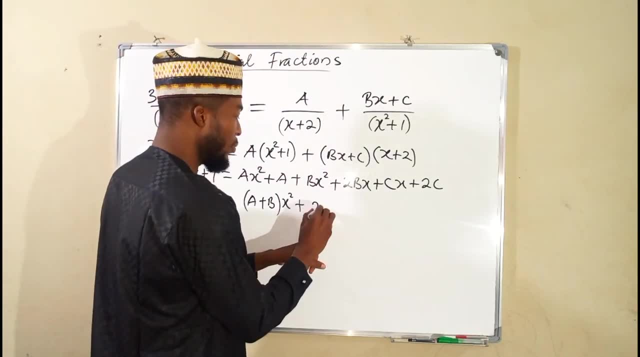 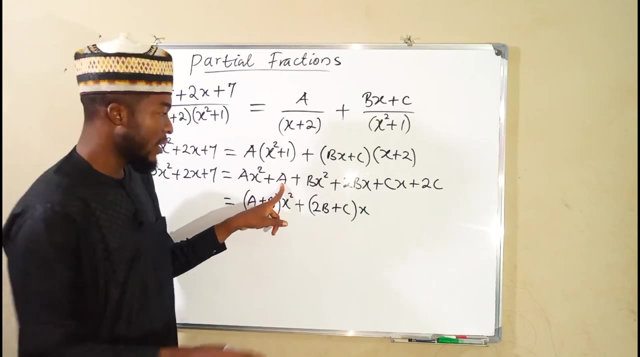 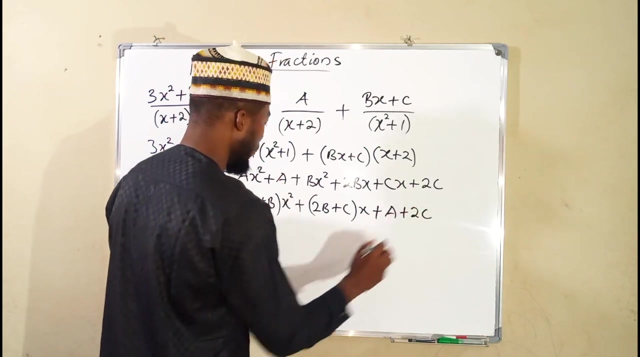 Then we bring x squared out, plus we bring those with x. We can see we have one here, and we have one here. So this is the same thing as 2b plus c. Outside we have x, and those without x, we have a, and we have 2c, plus a plus 2, 2c. 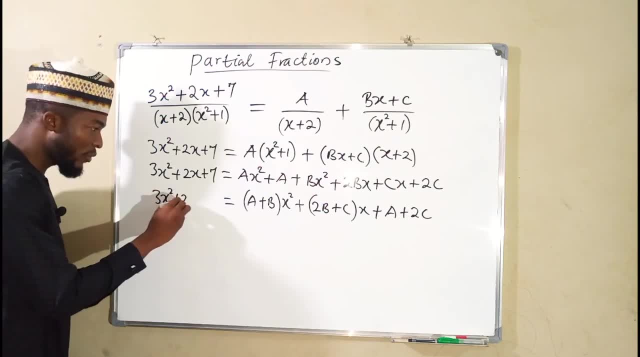 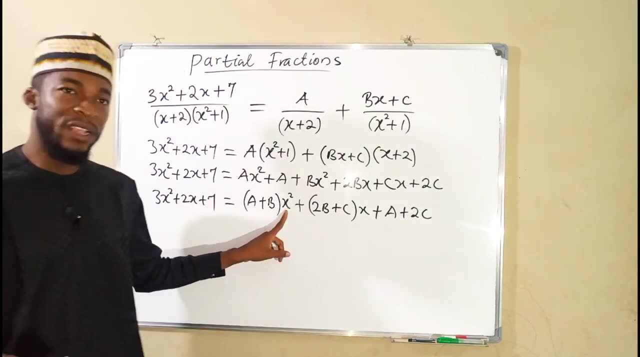 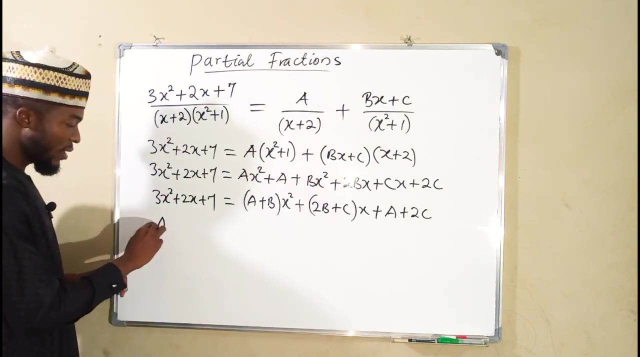 To the left we have 3x squared, plus 2x, plus 7. Therefore we are going to relate their coefficients. The coefficient of x squared to the right is just a plus b, while the coefficient of x squared to the left is 3. So we say a plus b is equal to 3. 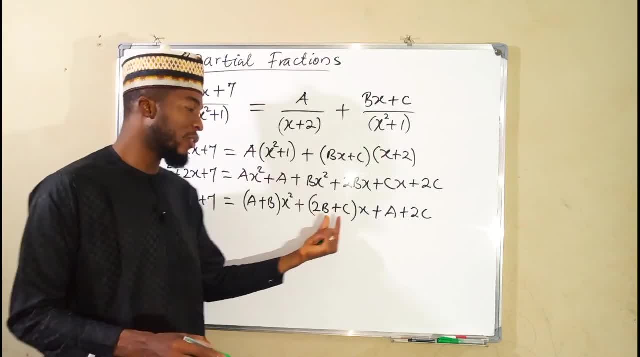 Those with x, we have 2b plus c. 2b plus c. 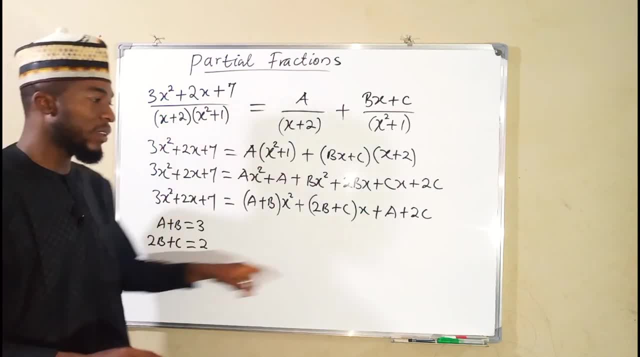 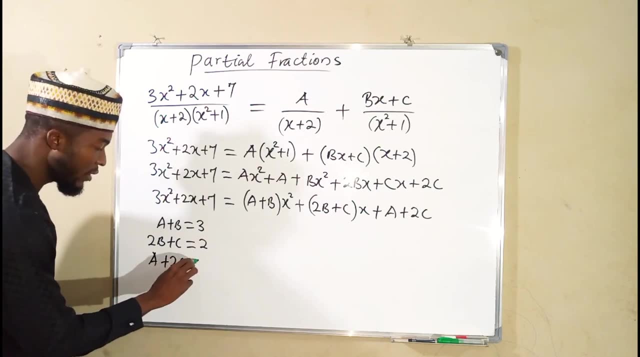 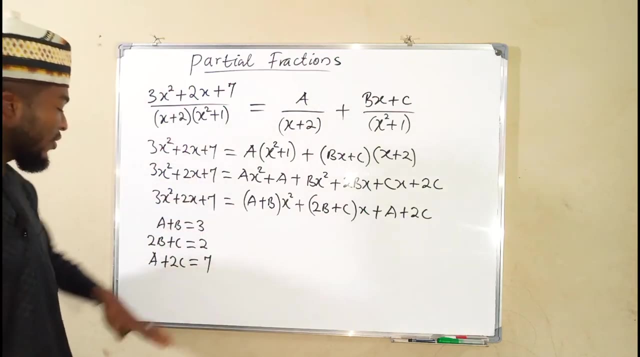 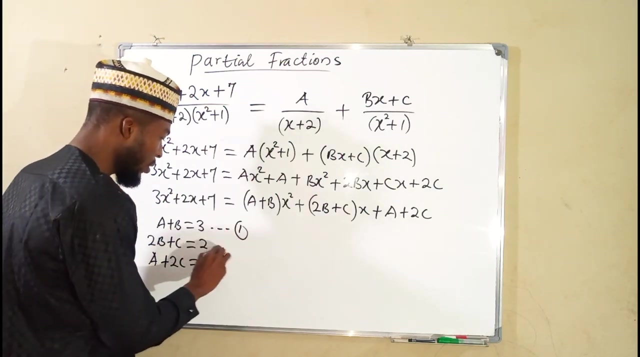 Must be equal to 2. And thus constant, a plus 2c. a plus 2c is equal to 7. These are the three equations we obtained by breaking these fractions down. We are going to solve them simultaneously. So let me name them. It's equation 1, equation 2, equation 3. 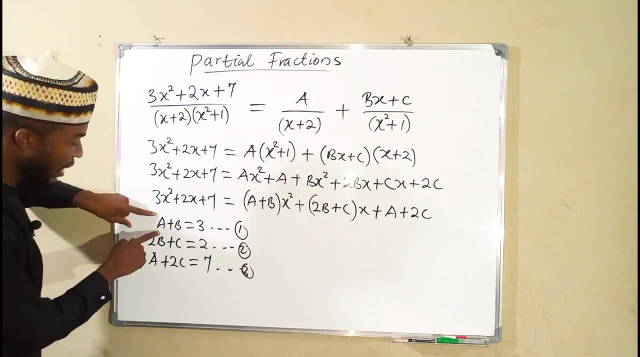 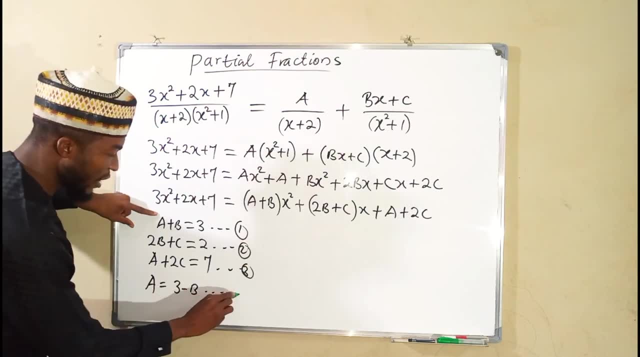 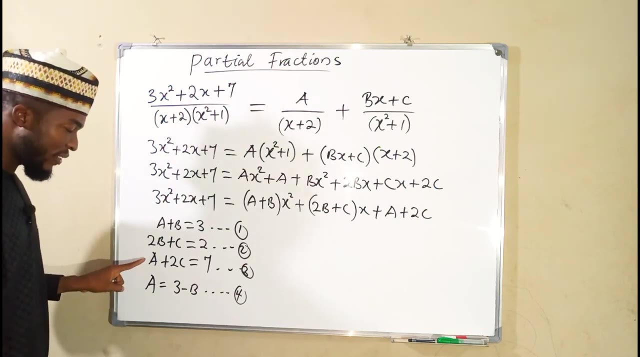 And from equation 1, we are going to solve them simultaneously. So from equation 1, you can see we can make a the subject. a can be equal to 3 minus b. And we can name this as equation 4. We obtain this equation from equation 1. And we can plug this into equation 3. By putting a into equation 3, wherever we see a, we replace it by 3 minus b. 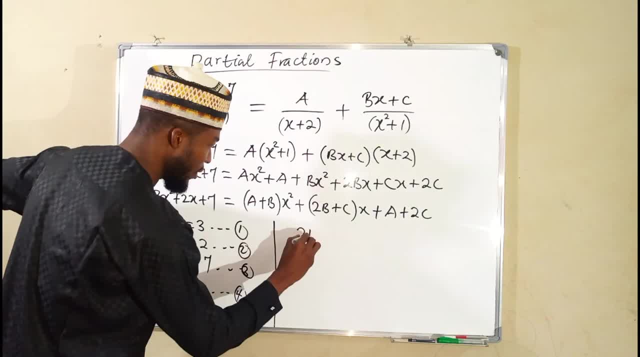 So let's repeat this one. We have 2b plus c. From equation 2. 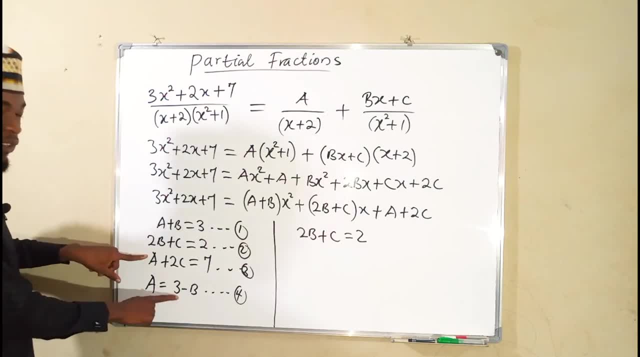 And from equation 3, if you substitute the value of a to b, 3 minus b, we have 3 minus b. 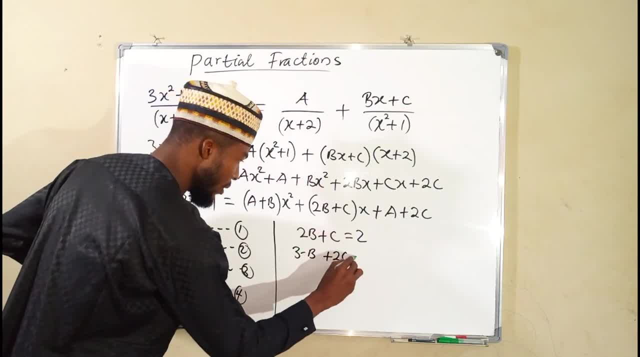 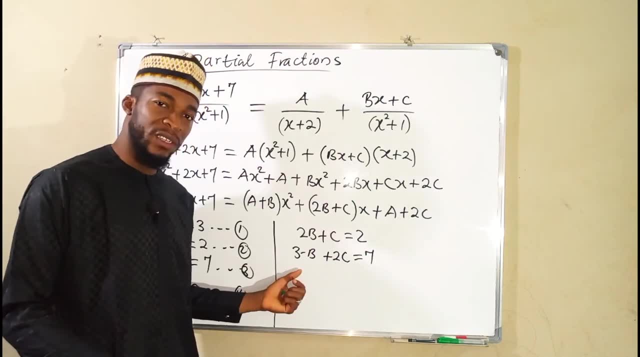 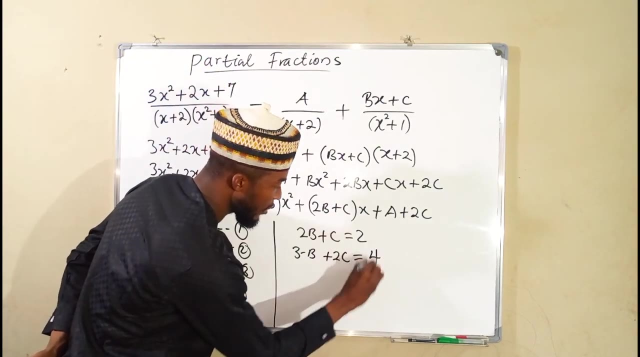 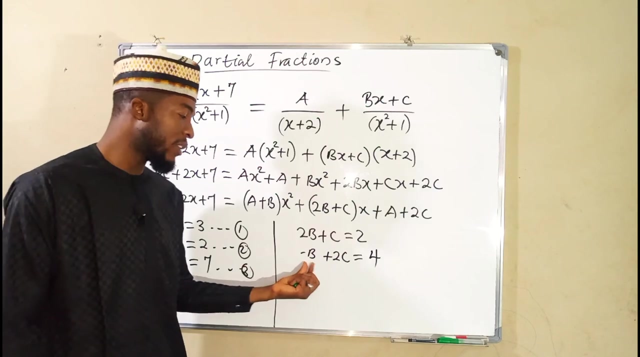 Then plus 2c is equal to 7. But we can take this positive 3 to the right by subtracting 3 from both sides. Minus 3 here, minus 3 here. We will have 4 here. And this will go. If we want to solve this simultaneously, we can multiply this equation by 2. If we multiply this equation by 2, we can eliminate b. So we say minus 2 here. This is 4. And this is going to be 8. 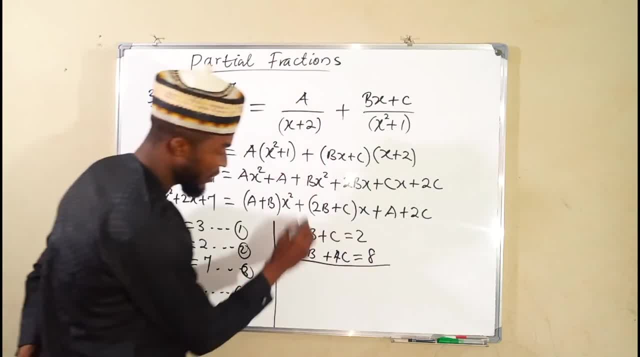 So now we can add these two equations together. This plus this is 0. This plus this is 5. So we have 5c here. This is equal to 10. 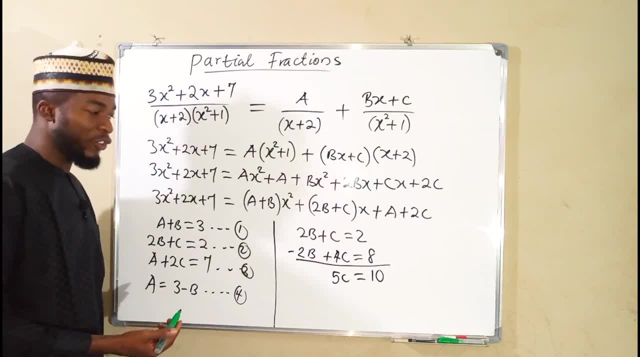 To find the value of c, we divide both sides by 5, which is the coefficient of c. c is now going to be equal to 2. 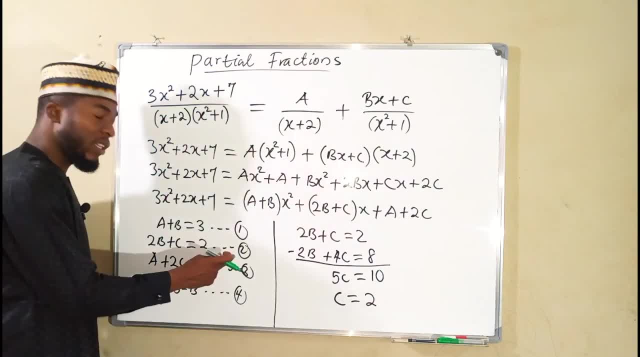 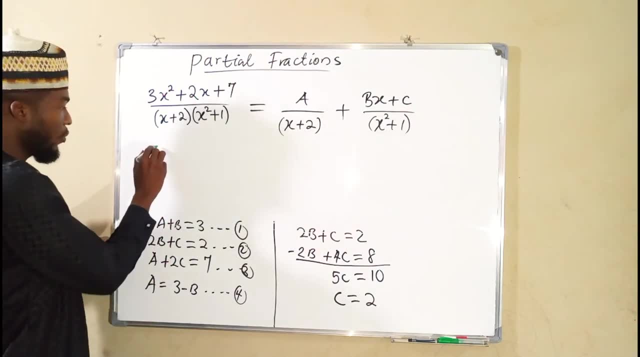 Having obtained the value of c, we can substitute it into equation 2 in order to find the value of b. From equation 2, we have 2b plus c equals 2. 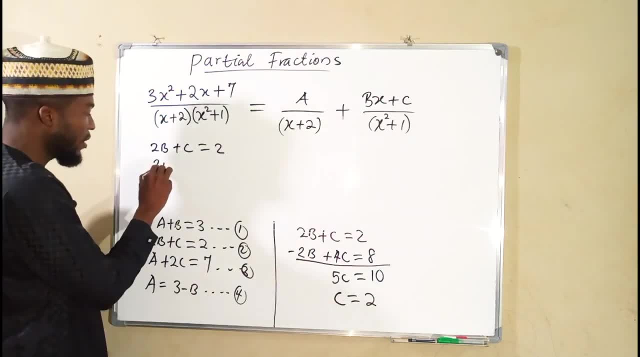 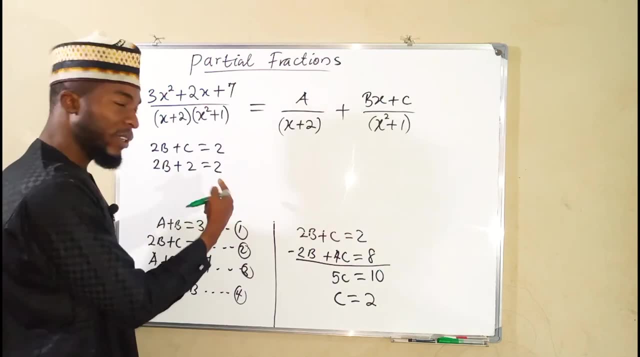 But c is now equal to 2. So we say 2b plus 2b. So 2 is equal to 2. If you take 2 to the right-hand side, it becomes negative, meaning 2 minus 2. We have 2b to be equal to 0. 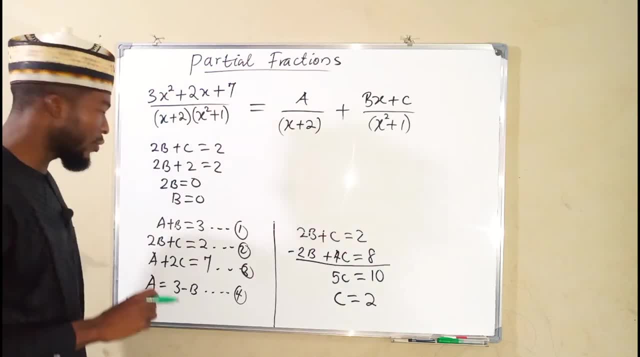 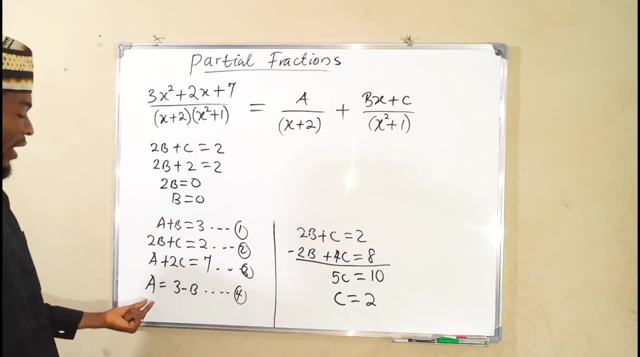 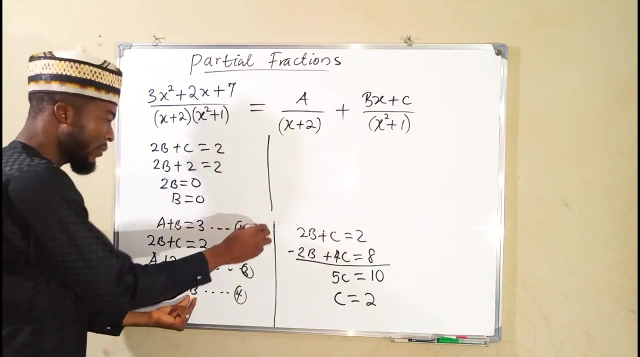 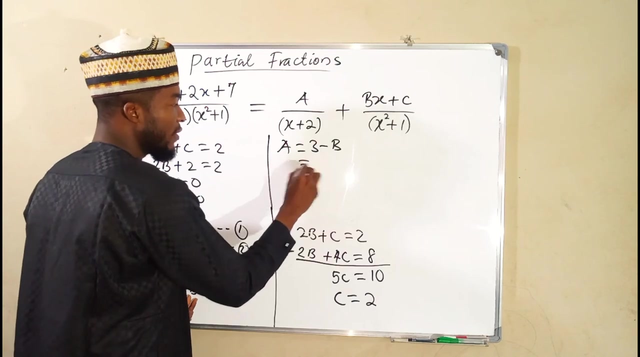 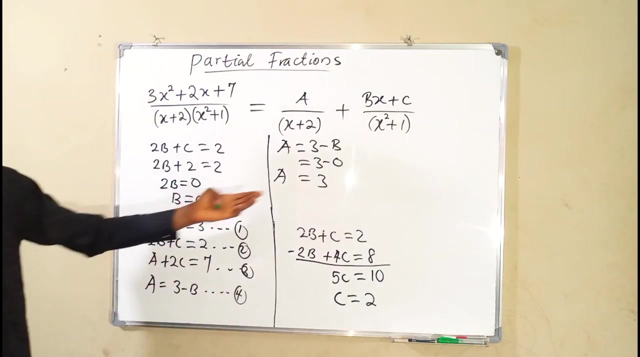 And b is equal to 0 if you divide both sides by the coefficient of b, which is 2. Now we have, of 10, b and c. We can find the value of a by substituting the value of b into equation number 4. So from equation number 4, you can see that a is equal to 3 minus b. And this is equal to 3 minus 0. And this is equal to 3. And hence, our a is equal to 3. Now we have obtained the values of a, b, and c. 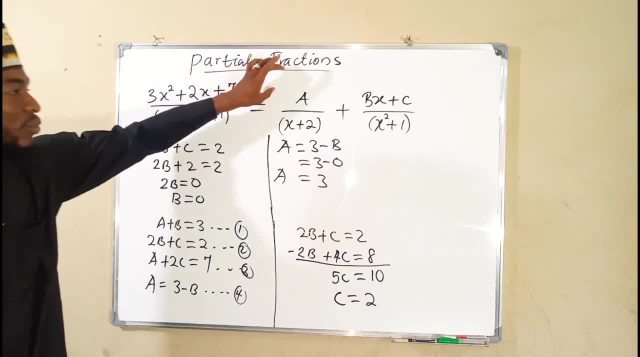 We can now substitute them back into this original equation in order to obtain our partial fractions. 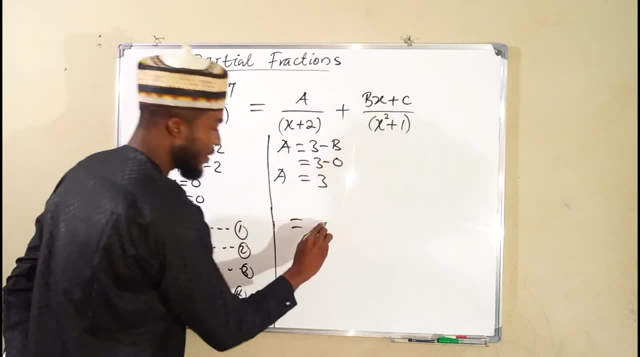 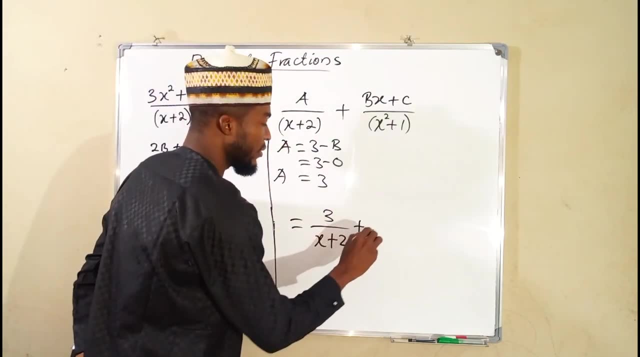 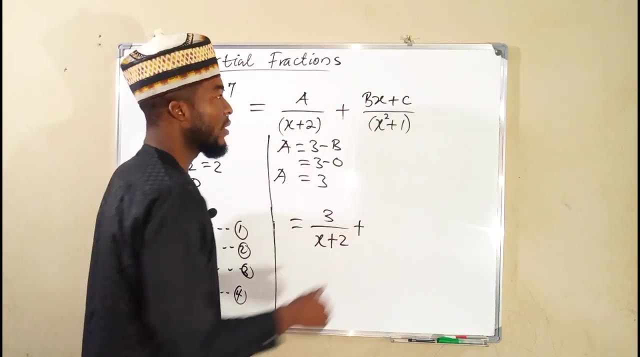 Our partial fractions are going to be, for a, we have it as 3. So we have 3. Over x plus 2. Then plus bx. The value of b is 0. 0 times x is still 0. What we have there left is just c. And the value of c, you can see it here as 2. 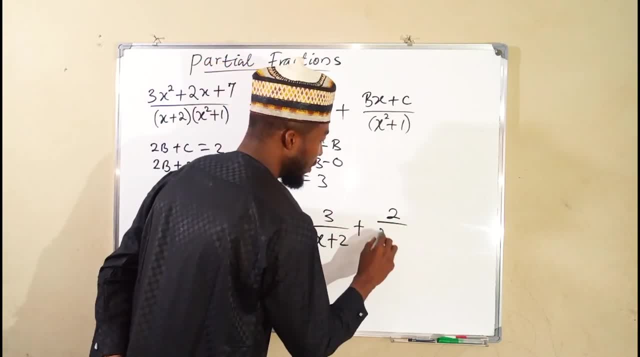 So what we have left is just 2 over x squared plus 1.